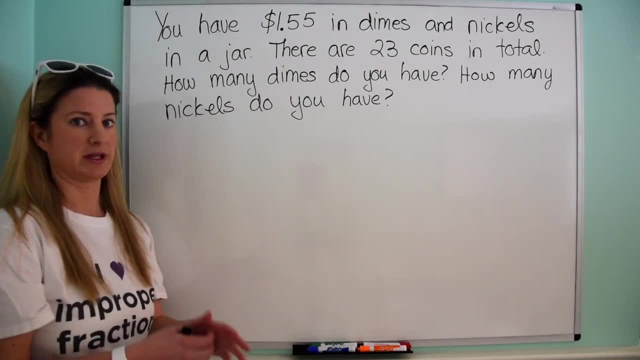 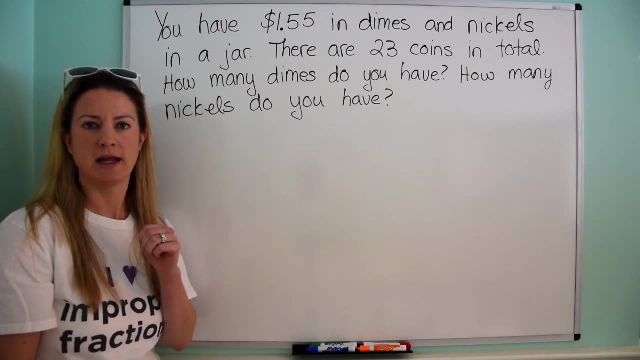 Now, when students see a lot of words, they get a little overwhelmed. typically okay, And I want to tell you that it's not that bad. Think about what this is saying. You've got $1.55.. You've only got dimes and nickels and you've got 23 coins in total. How many dimes do you have? How many? 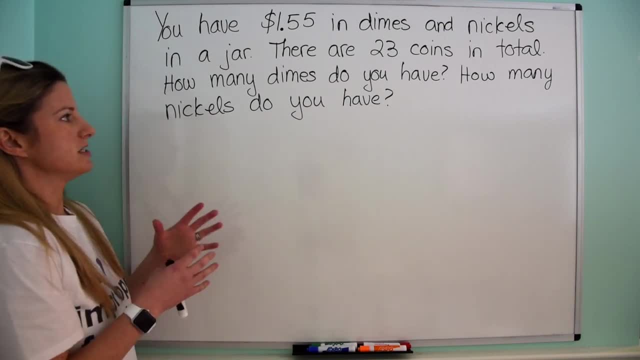 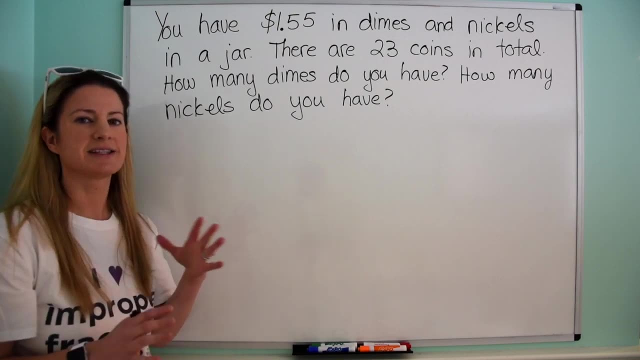 nickels do you have? That's what it's saying. So if you look at this, you're going to see that I don't even know where to begin. I understand, but there's clues, But usually, and I can't say this, 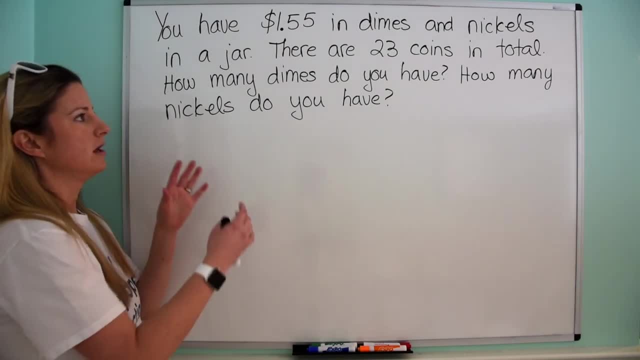 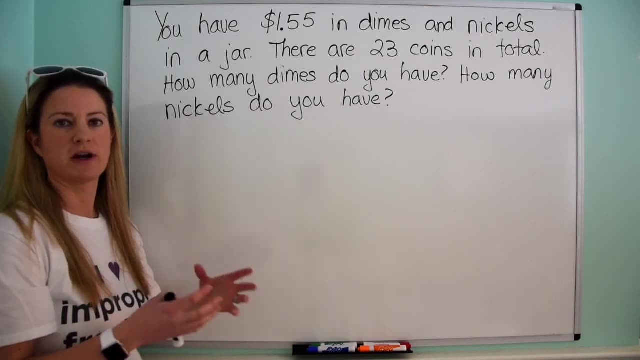 for sure 100% of the time, but the vast majority of the time. the last sentence- and it's the sentence that's going to have the question- is going to tell you what your variables are, And if you label your variables immediately, it makes the problem easier to solve. So let's take a look. 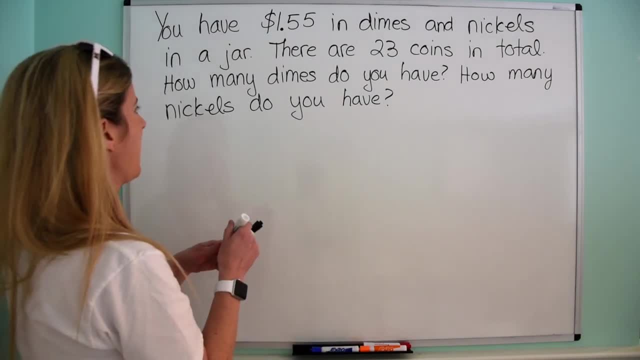 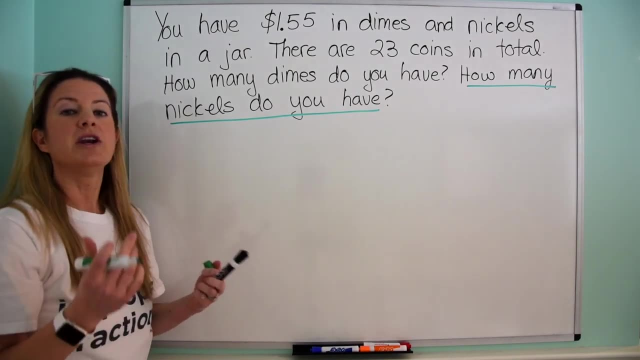 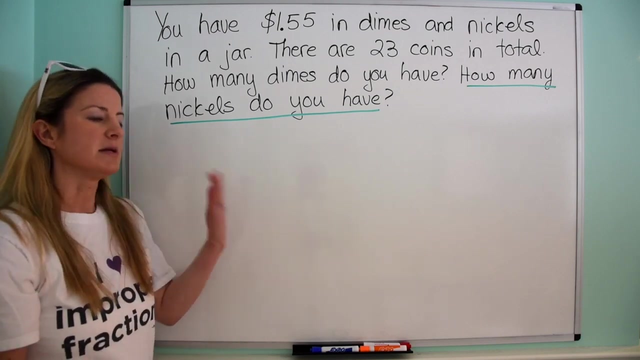 at this. What does the last sentence say? Okay, how many nickels do you have? How many nickels do you have? Well, if you want to know how many nickels you have, you know one of your variables is going to be number of nickels. Now, some students like to use x and y all the time. I personally like my. 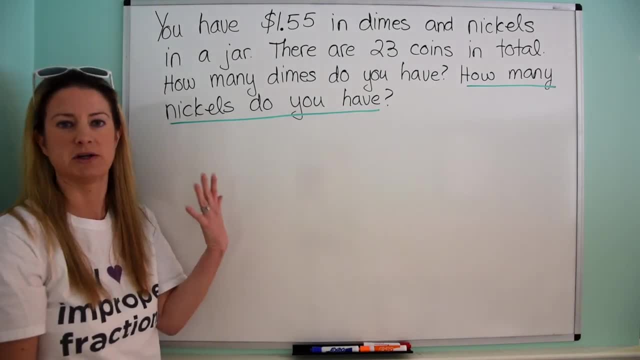 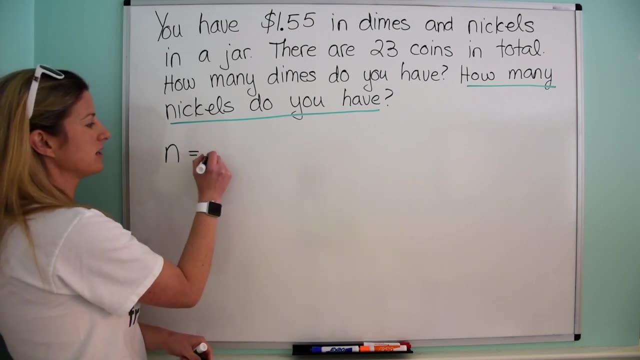 variable to kind of match with what I'm solving for, because for me it helps me to remember it better as I'm working through the problem. So I'm going to use the variable n and I'm going to say that n equals number of nickels. okay, 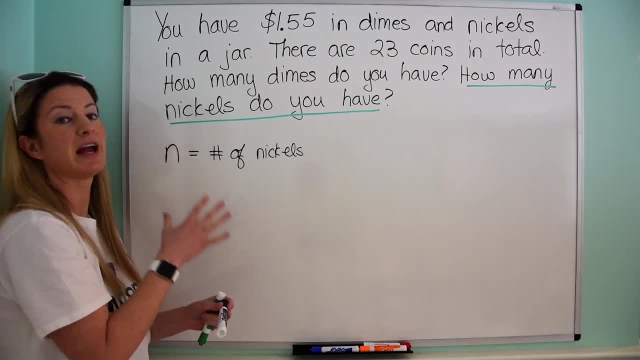 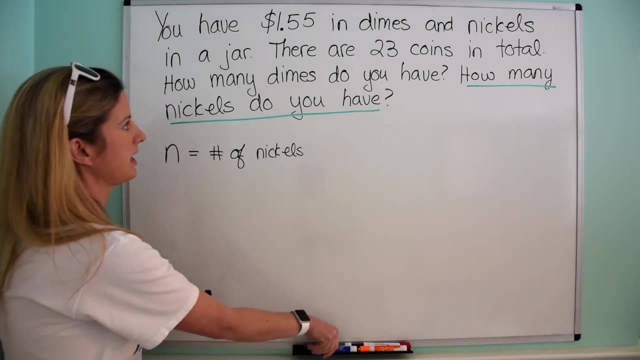 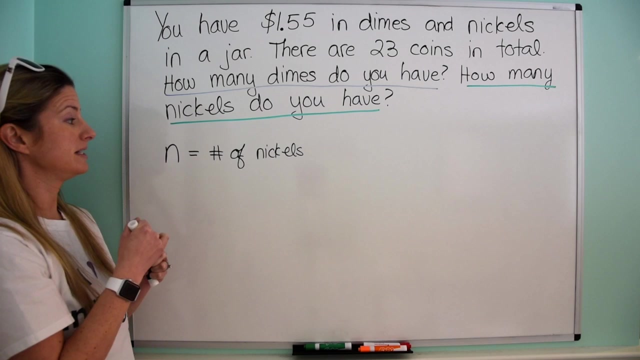 n equals number of nickels. And yes, don't do this in your head, Actually, write it out, okay. Now do I have another question in here? I do, And that other question is: how many dimes do you have? Okay, how many dimes do you have? So that's telling us that my other variable, 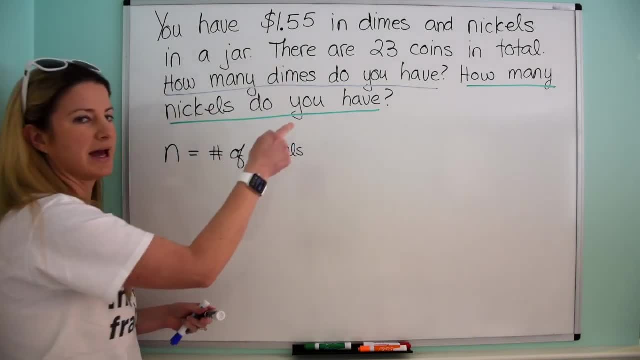 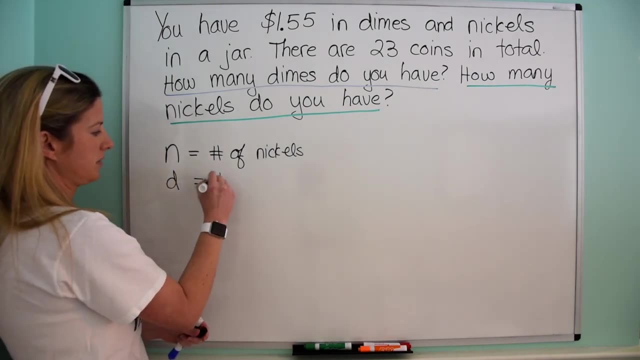 is going to be number of dimes, because it says how many dimes. So what's the variable, The number? I'm going to call it d, okay, Number of dimes. okay Again, if you call this x and you call this. 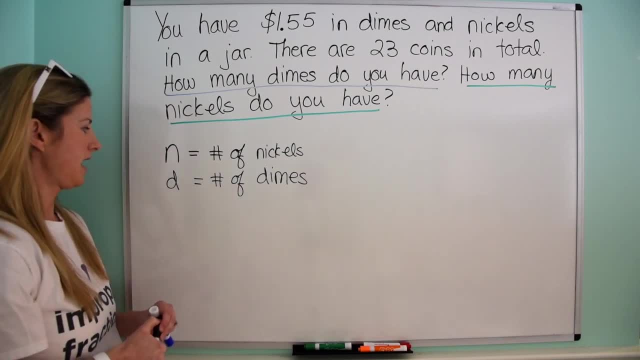 y. that's fantastic, and you do that For me. personally, I like to see n and d, because it makes my life easier. Okay, so now that we know our variables, it becomes very easy to figure out what our two equations are going to be. So we're going to look for the other data that we have. 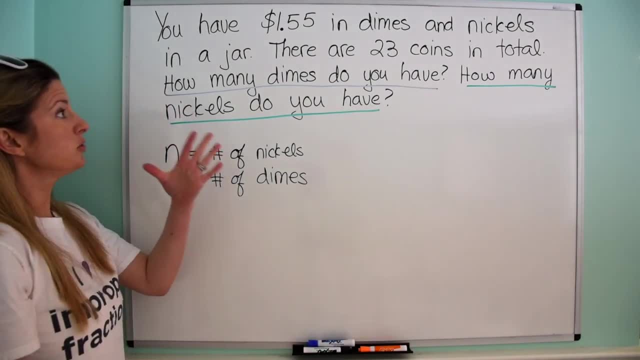 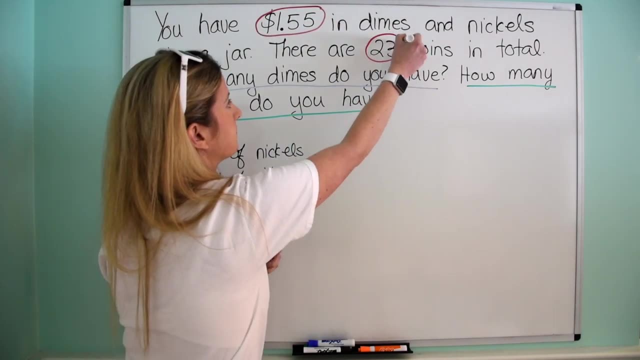 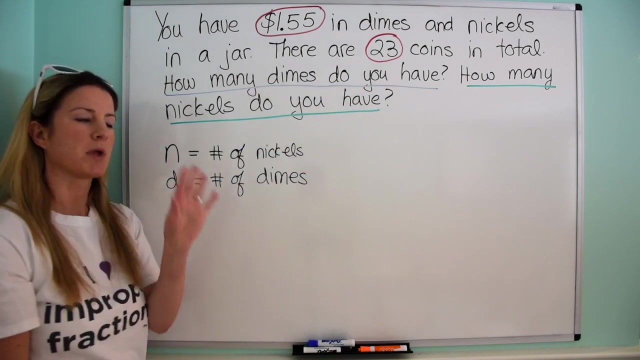 And if I look at this question here, I see two numbers that are jumping out at me. The first number is 155, and the second number is 23.. Okay, so let's see what those mean. So there are 23 coins in total. Okay, so, let's just stop for a. 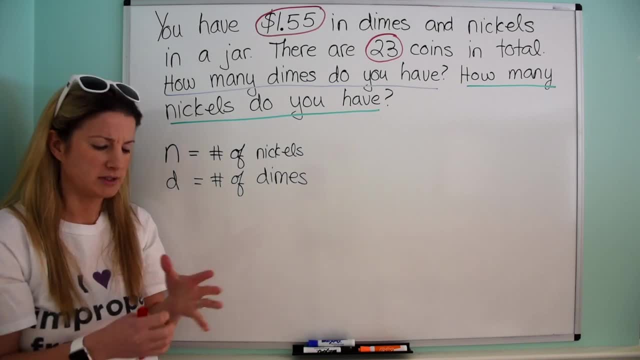 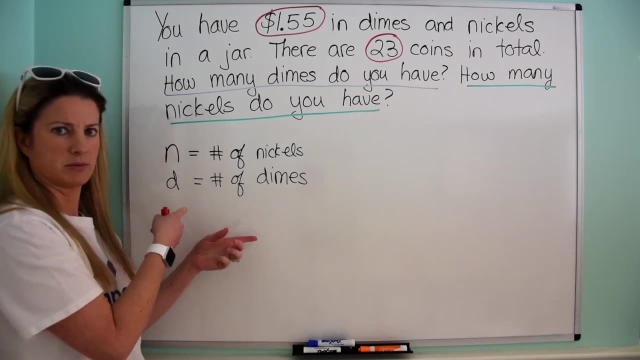 second and think about this: I have 23 coins in total. Okay, so if I'm putting out all the coins on the floor, I'm saying there's 23 of them. Now let me look at my variables: Number of nickels. 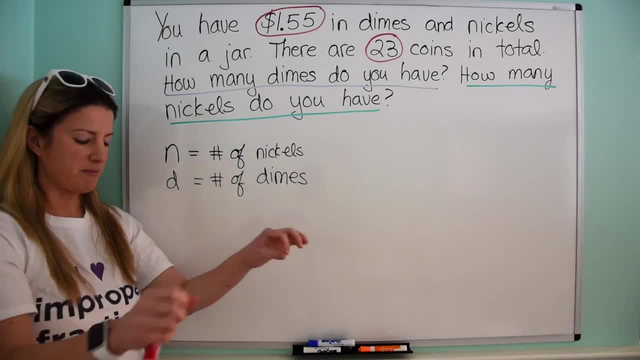 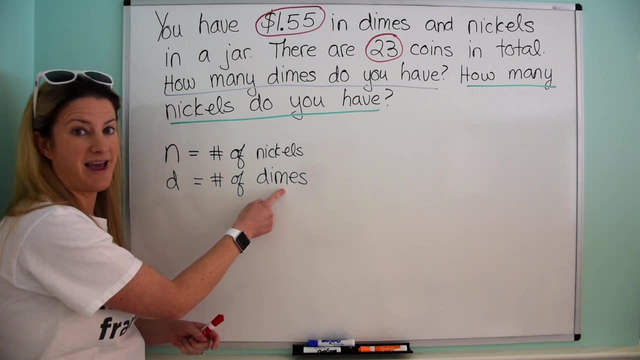 and number of dimes. Huh, So if I'm putting all my coins on the floor, I know I have 23.. That means the number of nickels I have plus the number of dimes that I have is going to equal 23.. So there's your first equation. 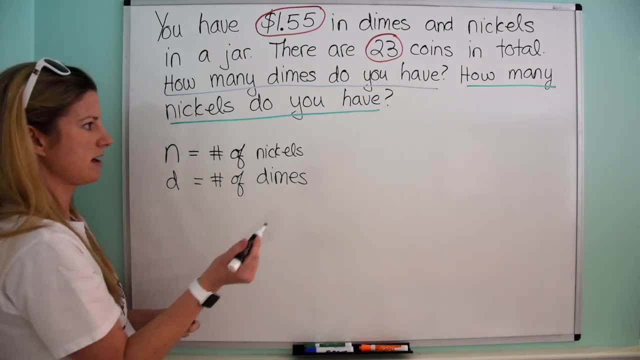 right there. Okay, so it's just going to be- I guess I'll write it down here: n plus d equals 23.. Okay, and we got that from the 23 up here, and then the fact that we labeled our variables. 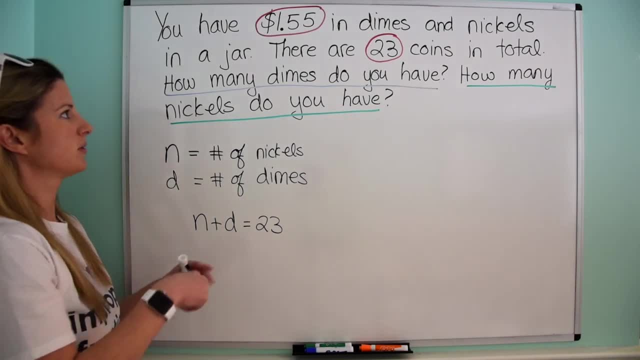 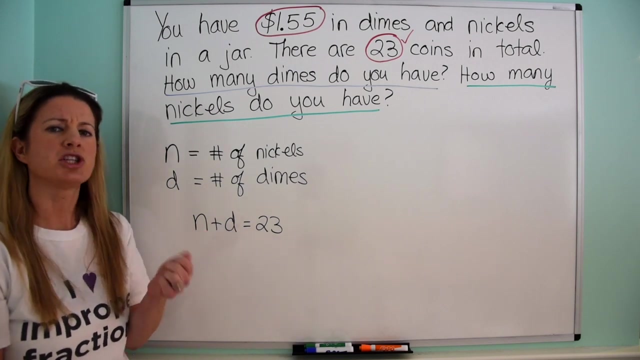 immediately. Okay, Now we've done the 23 piece, so check. Now let's look at the 155.. Okay, so 155 is going to be the value of the coins that I have right. So think about it. How much is a dime worth 10 cents or? 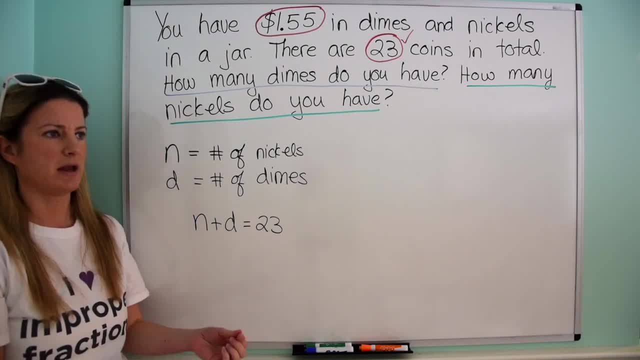 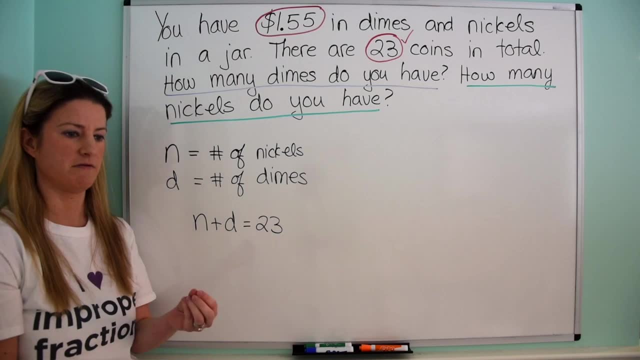 $0.1, right. So if you think about it, the amount of dimes I have, if I multiply that by 0.1, okay, that will give me The dollar value for the dimes that I have And the same with the nickels, except it's 0.05.. 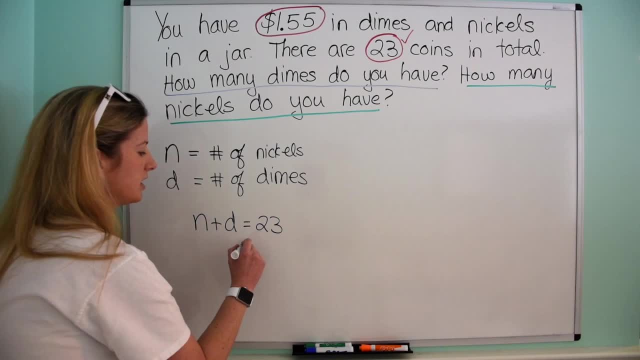 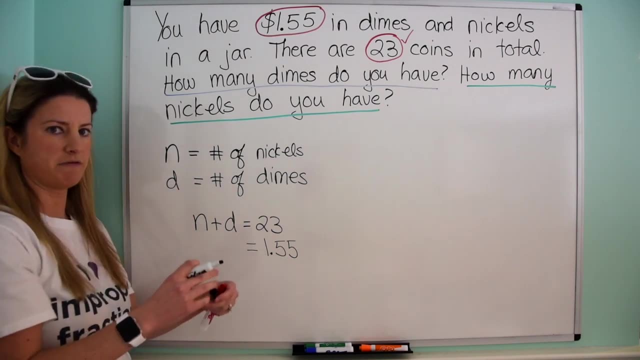 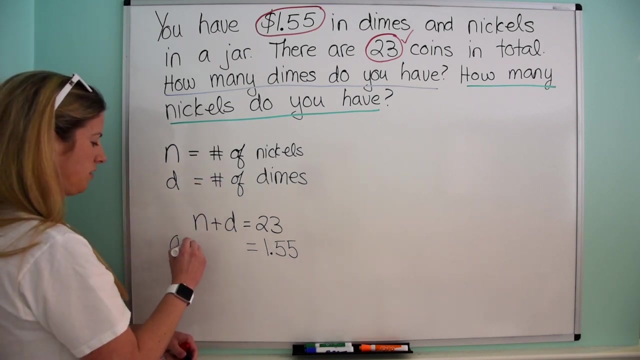 So I know that it's going to equal 155.. Okay, $1.55.. And I can say to myself: well, if I take 0.05, five cents, okay, 0.05, and I multiply it by the number of nickels I have, so 0.05 times. 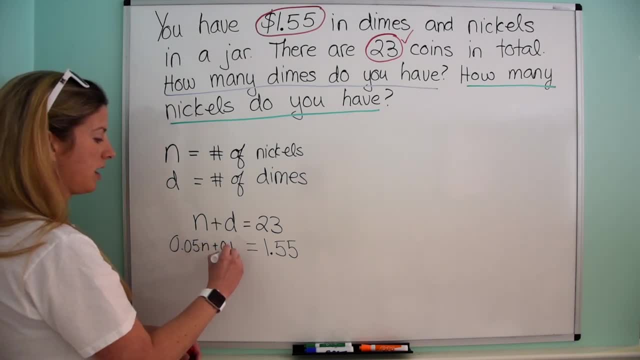 the number of nickels I have, plus 0.10 times the number of nickels I have. that's going to be the number of dimes that I have. You know what? I'm just going to erase that and make it a little. 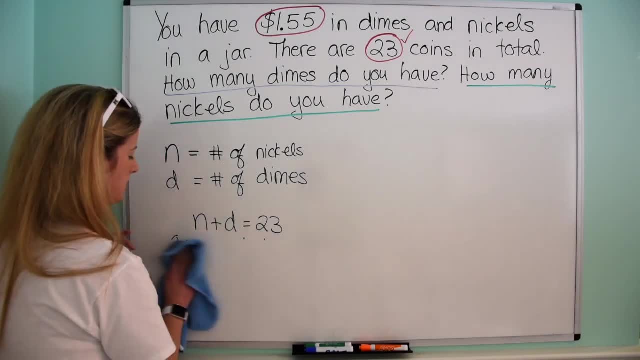 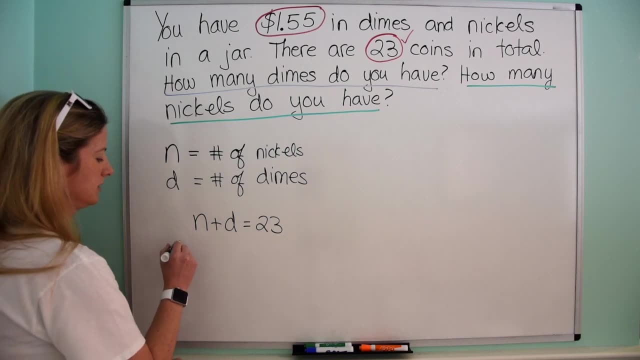 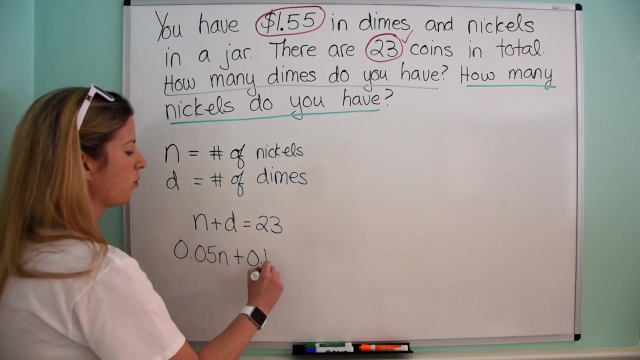 bit bigger so we can see it better, just in case. So let me erase that Okay. So again, if I say I've got 0.05 times the number of nickels that I have, okay, plus 0.10 times the number of dimes. 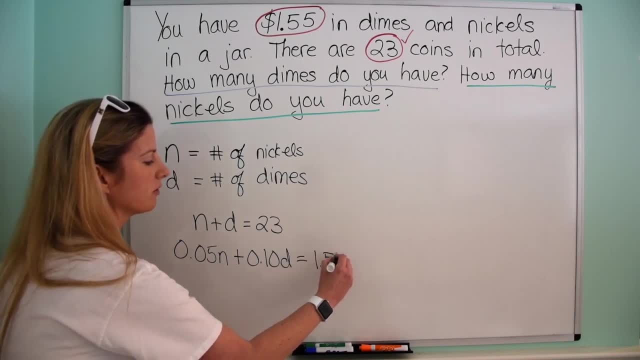 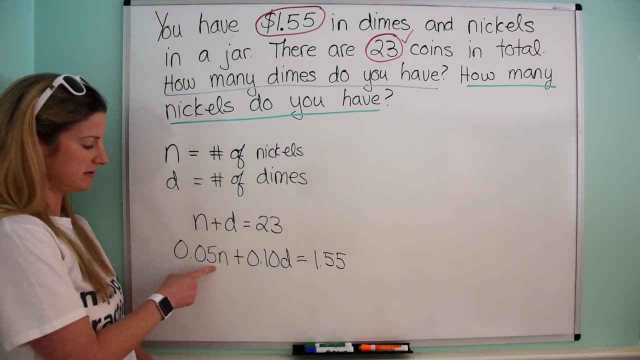 that I have. that's going to give me the total value okay, Of the coins, because each nickel's five cents Okay. So, for example, if I have 20 of them, I know I have a dollar and each dime is 10 cents. So I know if I have 10 of them I have a dollar. 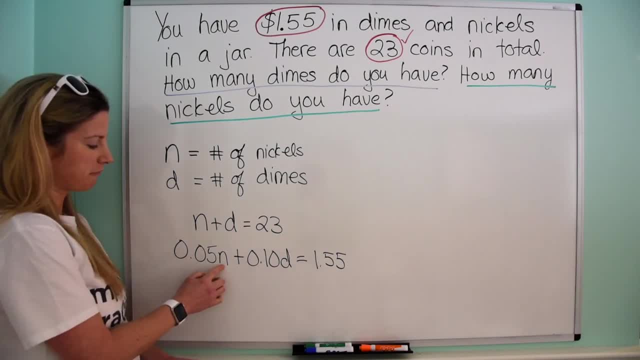 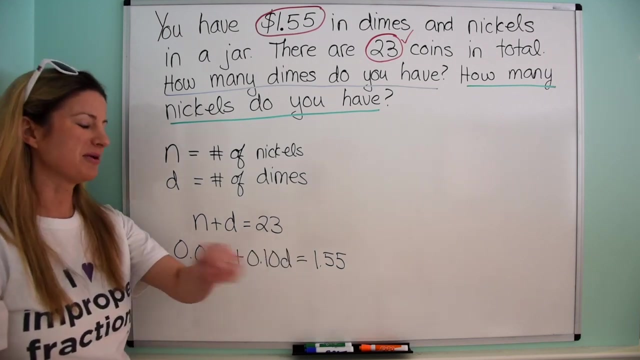 for example: Okay, So what you're placing in front of the number of nickels is it's just the value of the nickel times the number that you have, the value of the dime times the number that you have. Okay, There you go, And this is cake now. Okay, Except the only thing I'm going to say. 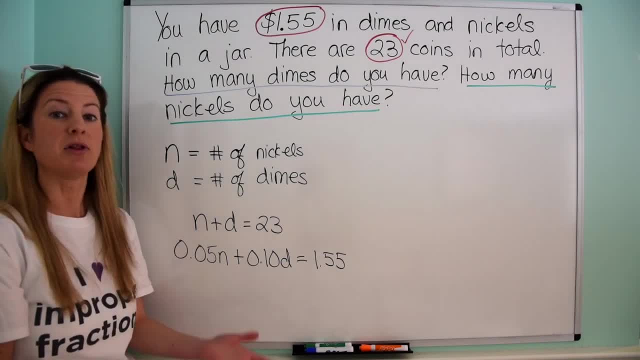 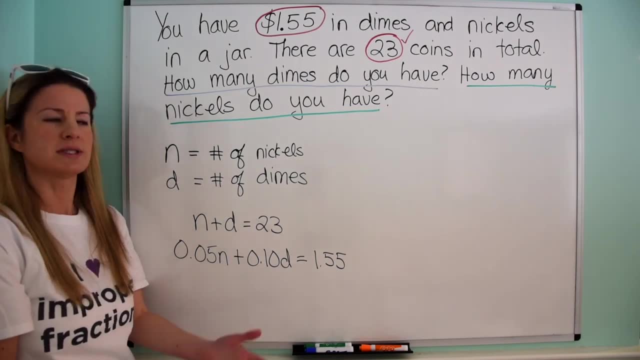 is: we're looking at this and we've got decimals. Okay, And how many people love decimals? I think decimals are cool, but I understand I'm not in the majority with that opinion, Okay, So I always tell students: if you don't like fractions or you don't like decimals, that's not a problem, You can just. 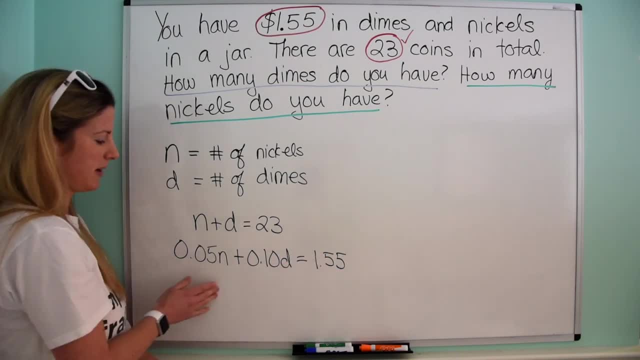 get rid of them. So think about it: If you multiply both sides by a hundred, you're going to move this decimal over. You're going to have five N, you're going to have one, two, 10 D, and this is just. 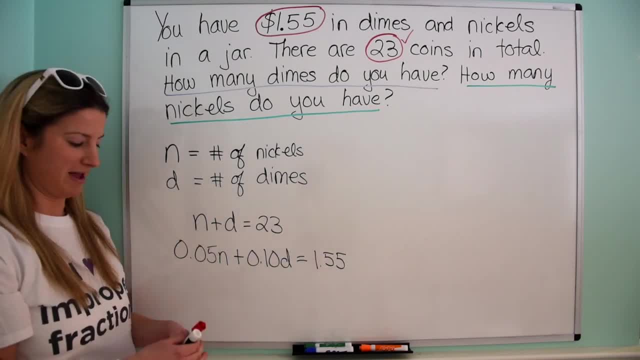 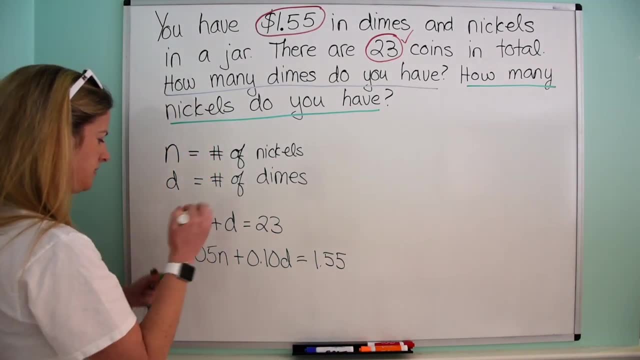 going to go to 155. So we might as well do that, because it's going to make our life a lot easier. Okay, So you don't have to do any extra work with all of these decimals. Okay, So I'm going to take. 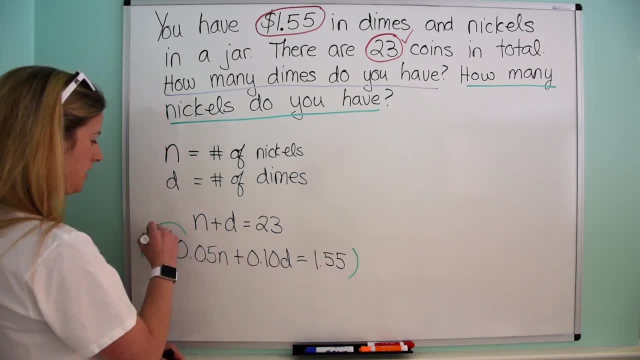 this: multiply it by a hundred, Okay, And always draw in your lines. I can't tell you how many students do this and forget to draw the lines, And then this gets multiplied by a hundred. Oops, they forgot that And they multiplied that by a hundred, Okay. So make sure you draw those lines. 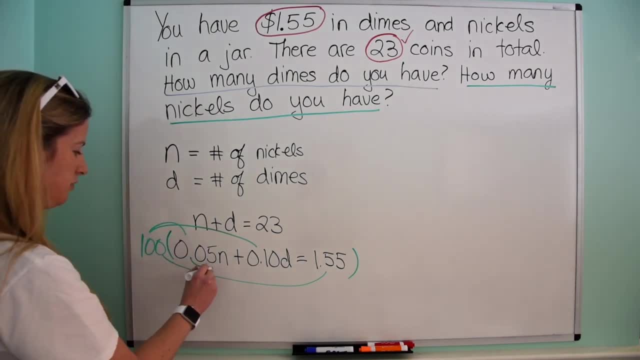 in: Okay, So a hundred times 0.05 is all I'm doing is moving the decimal point. So that's just going okay. And again move the decimal point one, two, that's going to be plus 10 D, Okay, And that's. 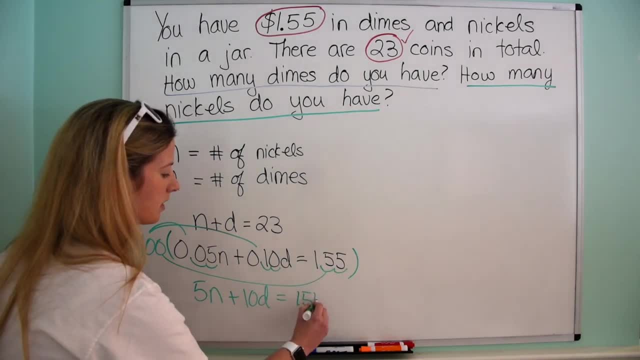 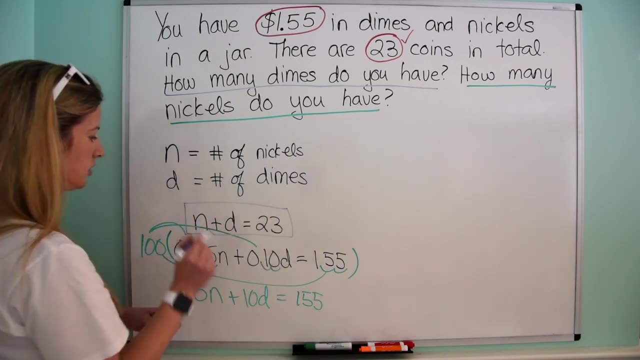 going to equal, move the decimal point one, two, 155.. Okay, So now I have my two equations and I know it's a little messy here, so I'll try to box them and then we'll move them. So here's my first. 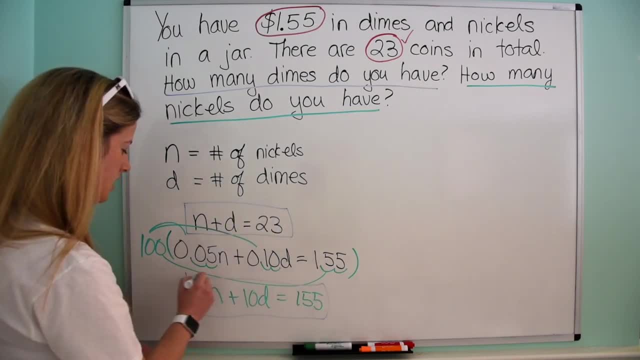 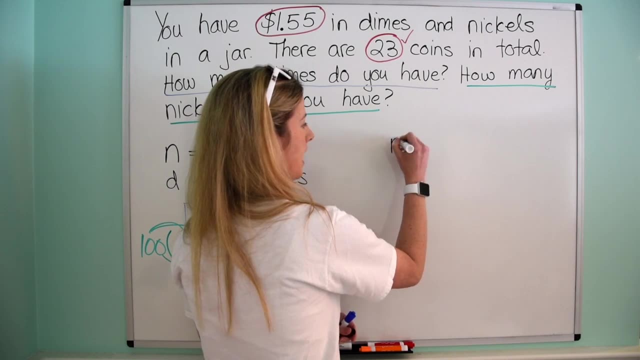 equation: N plus D equals 23.. And here's my second equation. Okay, Five N plus 10 D equals 155.. So why don't we come up over here and do that? Okay, So N plus D equals 23.. 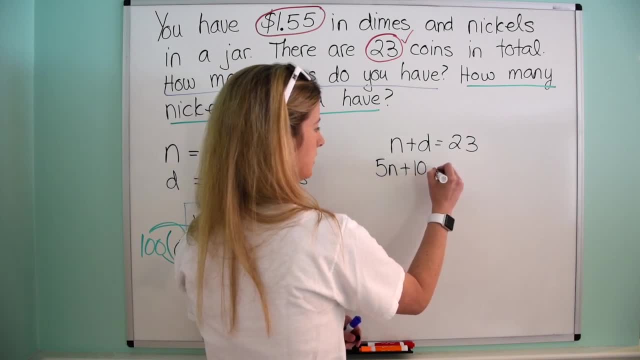 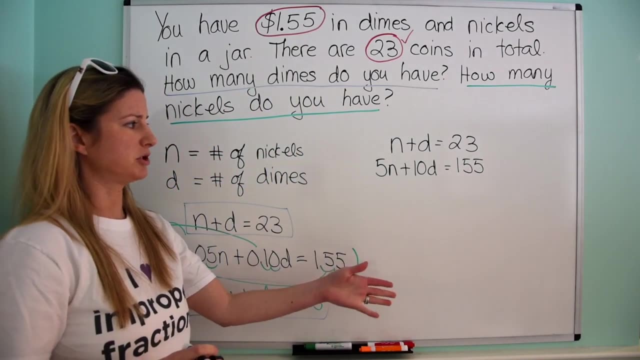 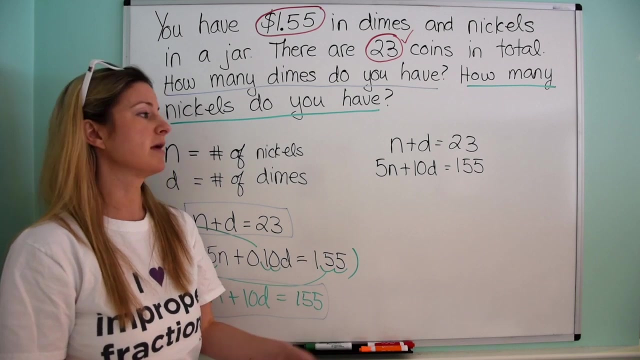 And five N plus 10 D equals 155.. Okay Now, at this point I have two options. I can solve by substitution or I can solve by elimination. Theoretically, I could also solve by graphing, but substitution or elimination will be the fastest way, since we're using a pen and paper. 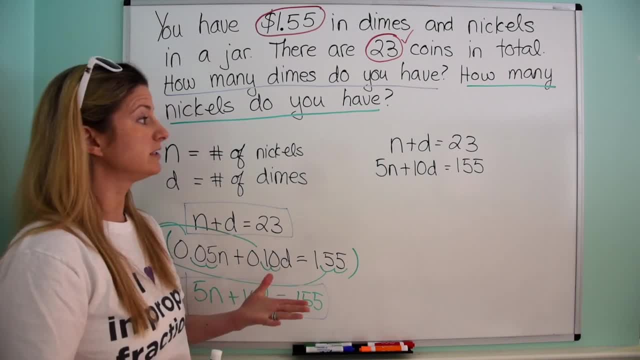 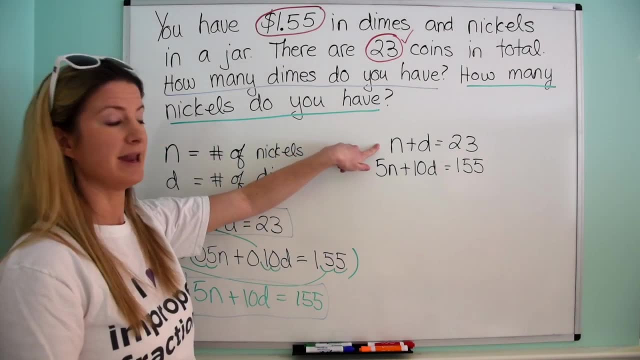 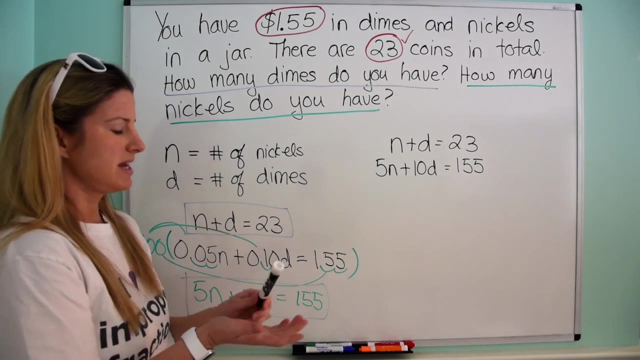 right now, or pencil and paper. Okay, So what I could do is I could multiply this by negative five or negative 10, depending on what I want to do. Okay, So let's say I were to multiply it by, I mean, negative 10 is probably the easiest. Okay, So I multiply this by negative. 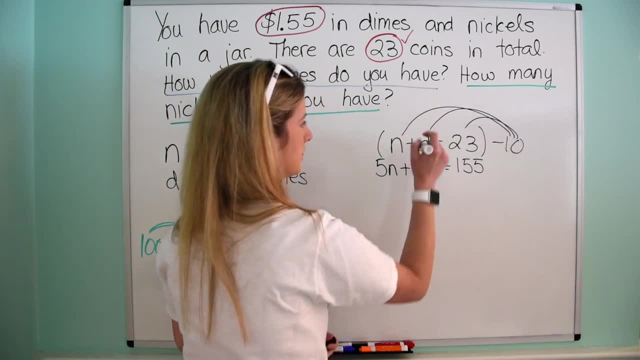 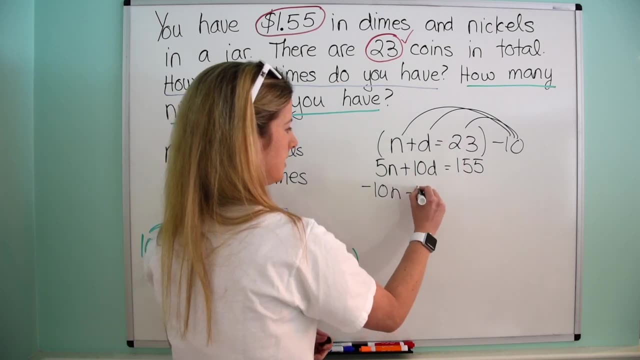 10. And again, draw those arrows, please. Okay. So negative 10 times N is just going to be negative. 10 N, Okay. Negative 10 times D is going to be minus 10 D, Okay. And then 23 times negative. 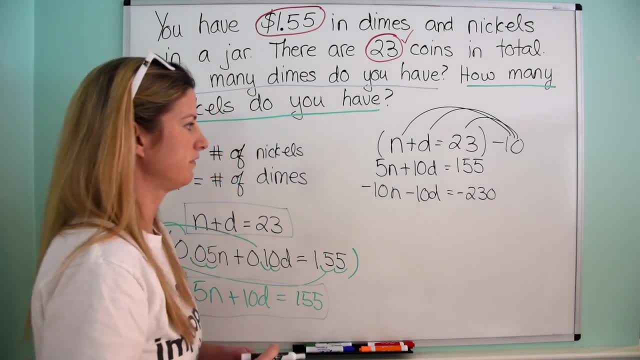 10 N is going to be minus 10 D. Okay, So I'm going to multiply this by negative 10.. And again, and it's gonna be negative 230,. okay, perfect, All right, now I just do the addition. 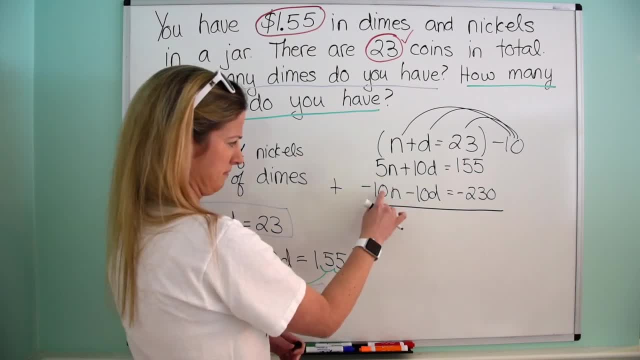 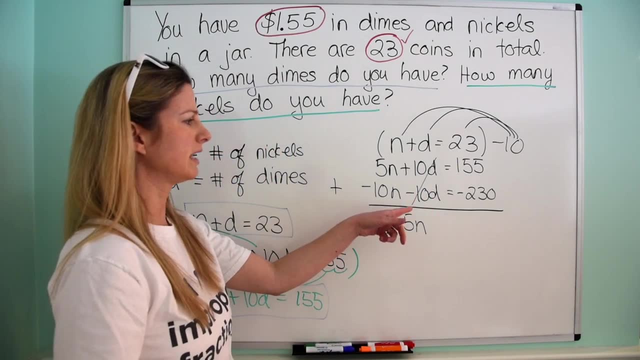 so five plus negative 10, so five n plus negative 10 n okay is gonna be negative five n okay. These go away. perfect. And 155 plus negative 230, so there's a couple ways to kind of think about this. 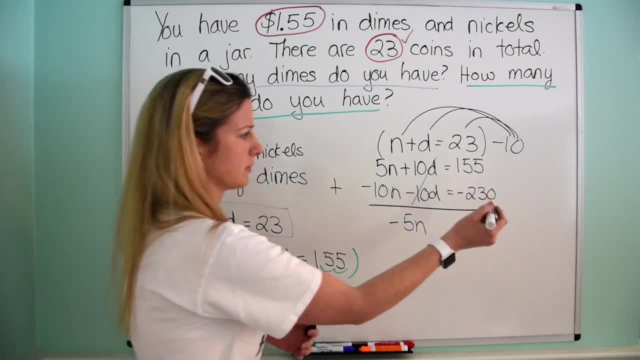 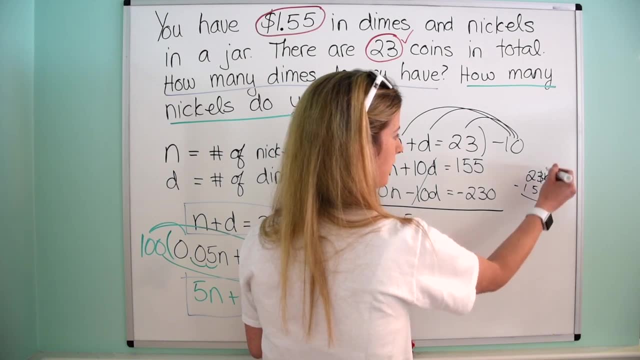 You could just do, you know, 155 minus 230, you could do 230 minus 155 and just know that it's negative. so if you were to do 230 minus 155, okay, so you borrow here you get: 10 minus five is five. 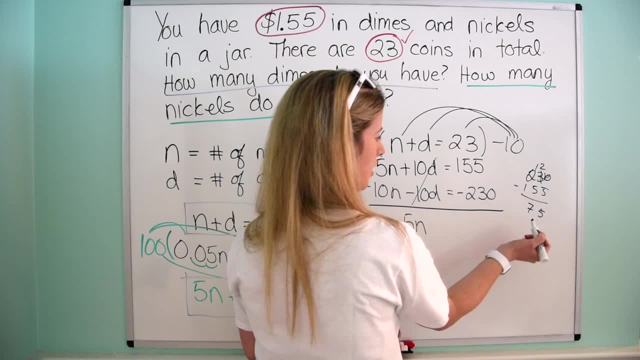 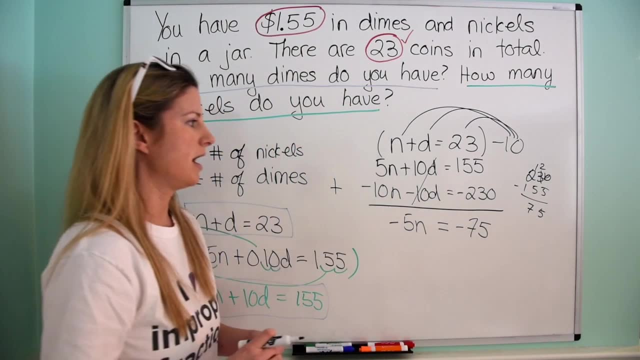 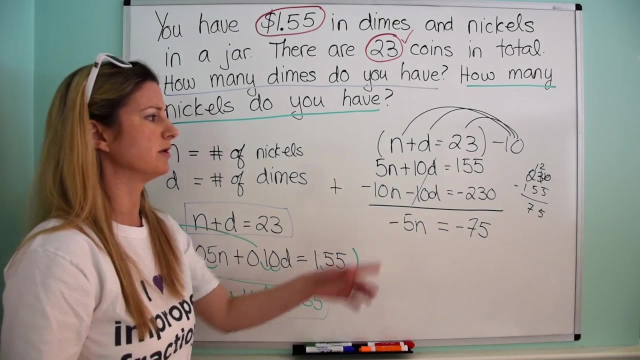 this becomes a two, 12 minus seven, and then there you go. So you know it ends up being negative 75,. okay, You could also just actually do the subtraction. you could use a calculator, you know. whatever you wanna do. however, you wanna do it. 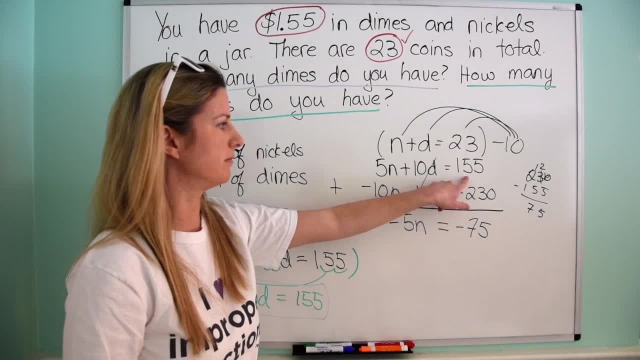 You can also solve by addition. you can say: how many do I need to get? from 155 to 230, and that's gonna be 70,, and that's gonna be 75, but then it's negative because you're going negative. you know what I mean. 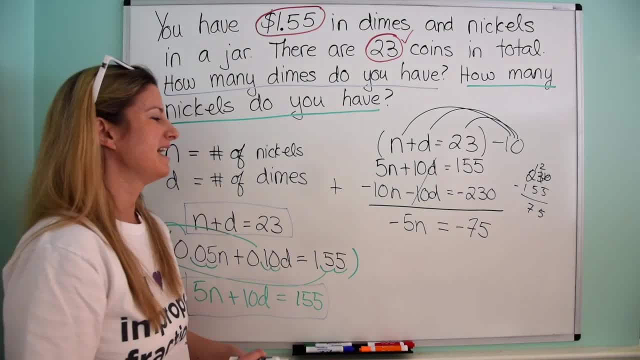 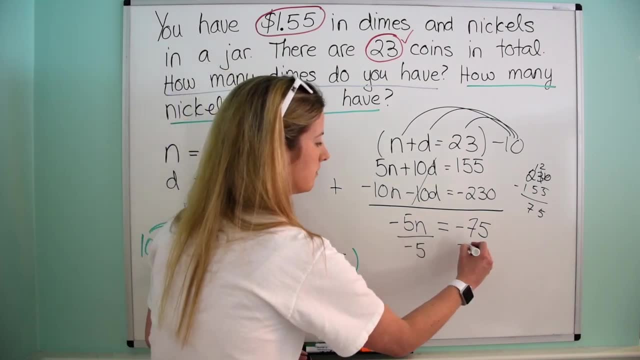 There's a lot of ways to do that, but of course, if you just wanna use a calculator, go for it, Okay. so now we have negative five. n equals negative 75, so we're just gonna divide by negative five. divide by negative five, okay. 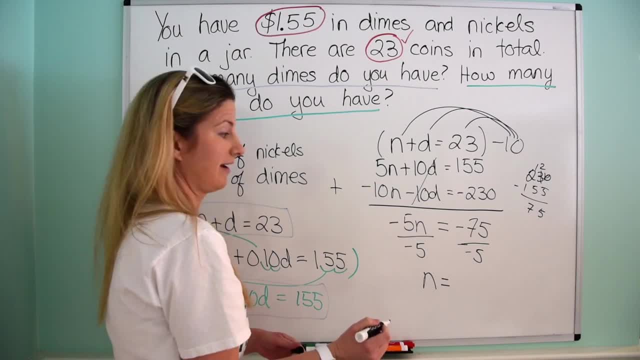 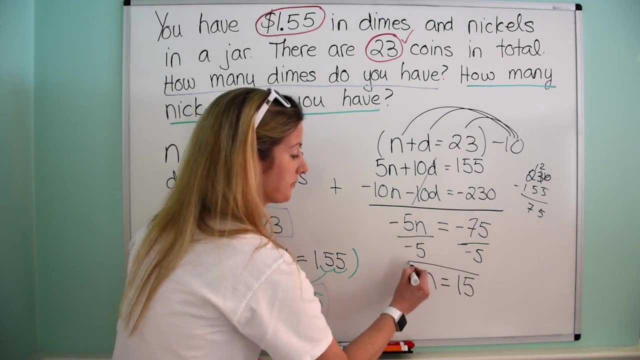 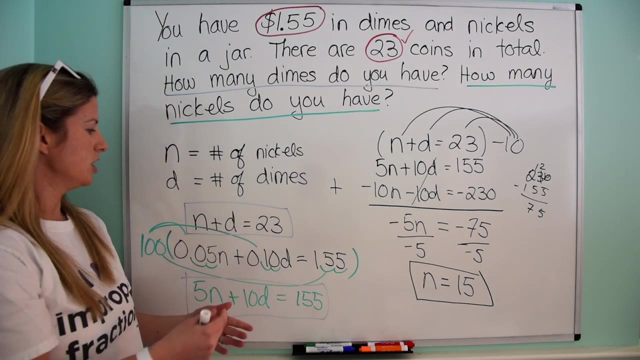 So then n is going to equal what? 15?? Okay, so n equals 15,. there you go. All right, so now I know the number of nickels that I have is 15, and now I wanna find the number of dimes. 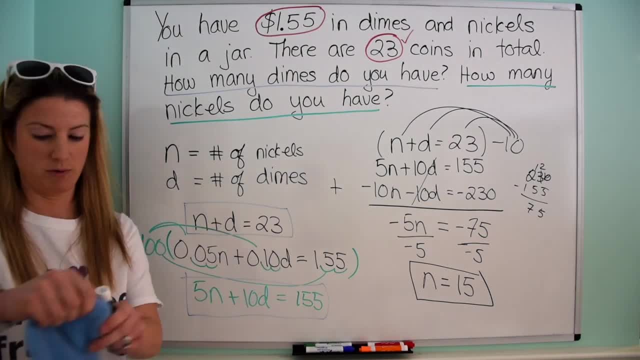 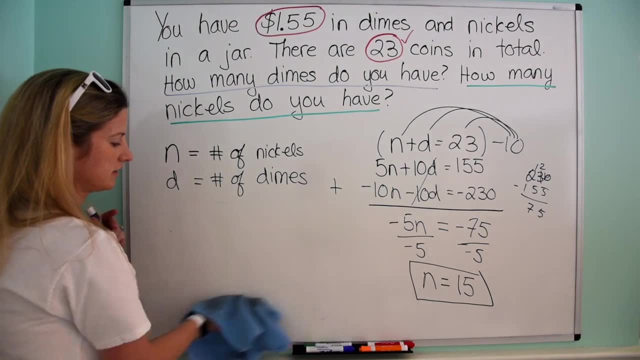 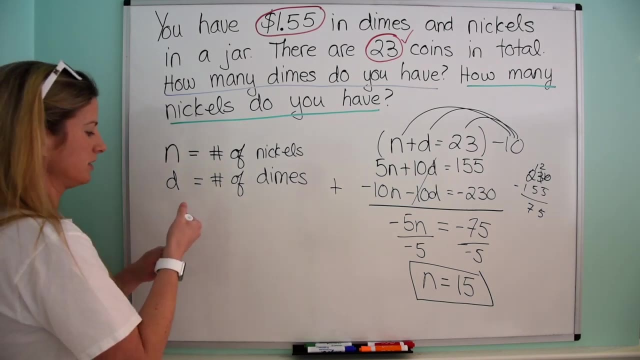 Well, this is super easy, because I'm gonna erase this over here just so I have more room. okay, I know that I have 15 nickels, Oh, so the question is, how many dimes do I have? And I say to myself: well, one of my original equations- 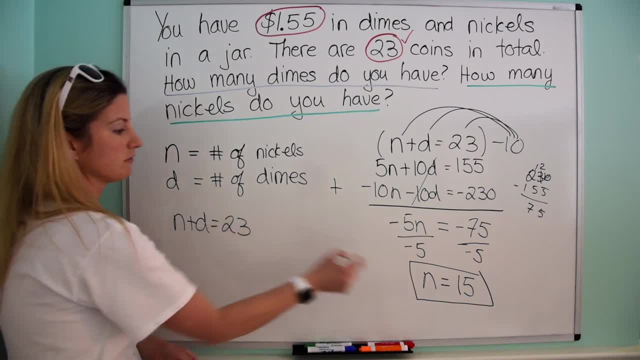 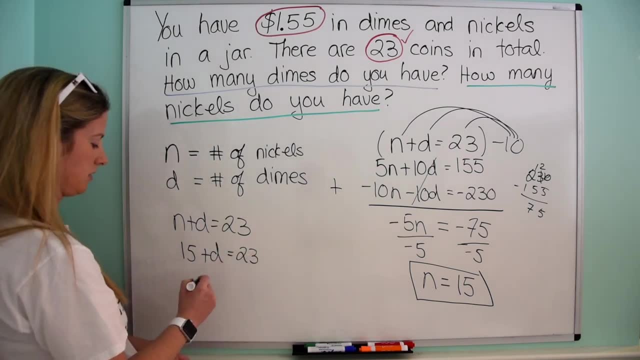 which I just erased over here, was n plus d equals 23.. So, if I know n is 15, I'm just doing 15 plus d equals 23,. okay. so 15 plus what will give you 23?? Well, that's easy: d is going to equal eight, okay. 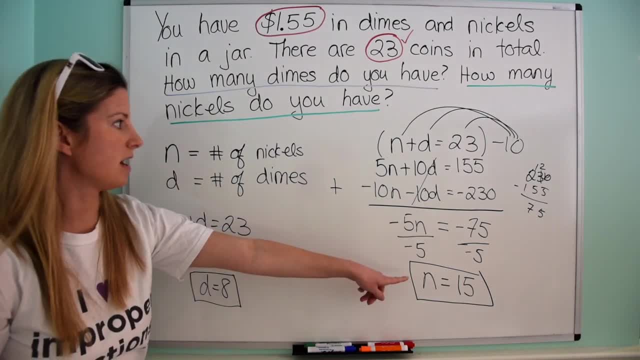 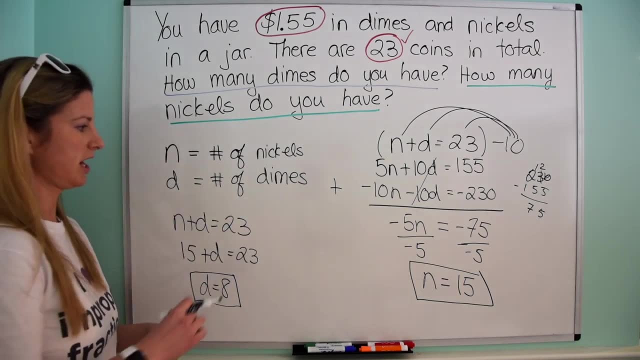 There you go. So you have now solved. you have 15,. what was it? 15 nickels, right, because that was n? yep, 15 nickels and eight dimes. Now, if you wanna double check, you can say: 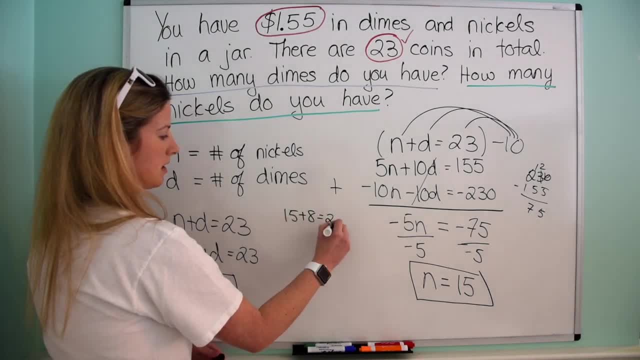 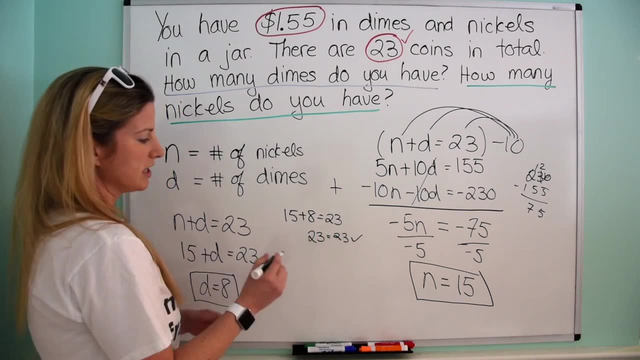 all right, is it true that 15 plus eight equals 23?? And that is true, 15 plus eight equals 23,. okay, 23 equals 23. Check. Okay, then you can check your second one, which is: is this $1.55??